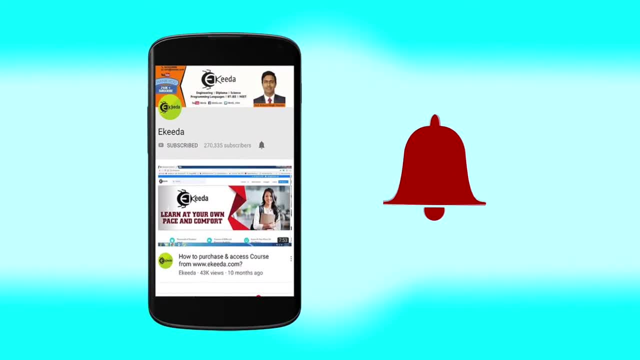 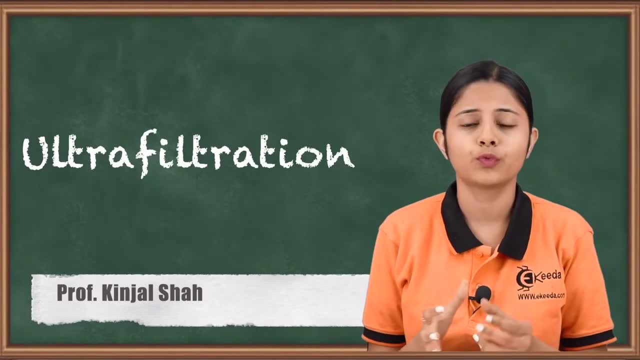 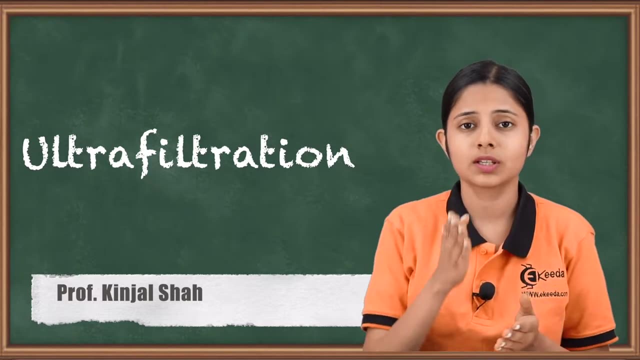 Click the bell icon to get latest videos from eKIDA. Hello friends, in today's session we are going to study one of the most important processes of purification of water, and that process is known as ultrafiltration. Ultrafiltration is a process which uses a semi-permeable membrane, but this membrane is different than the other. 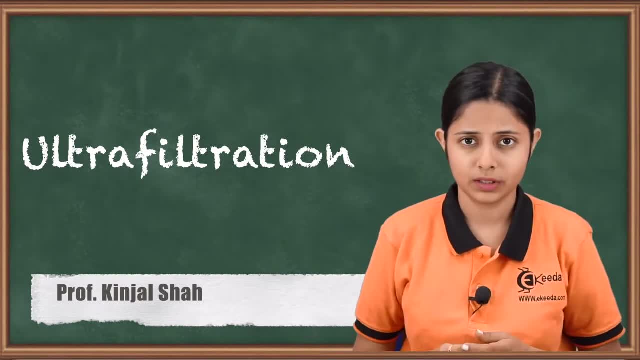 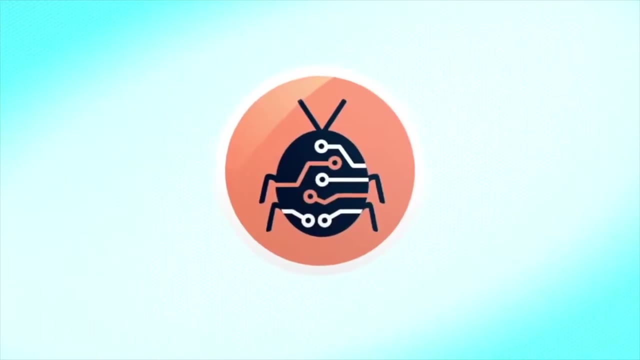 membranes. Many processes use a semi-permeable membrane. Hyperfiltration uses it, reverse osmosis uses it, but for ultrafiltration we use a special membrane. We will study about this membrane and we will study about this process in detail in today's session. Ultrafiltration is also known. 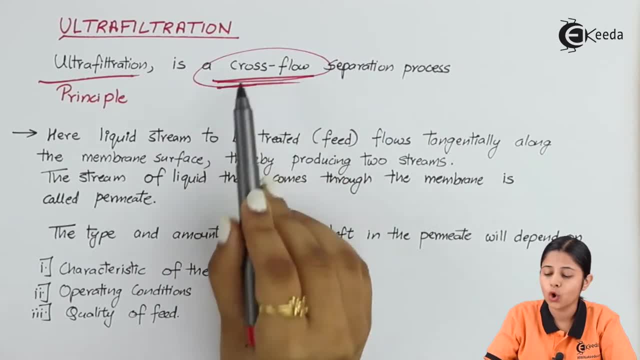 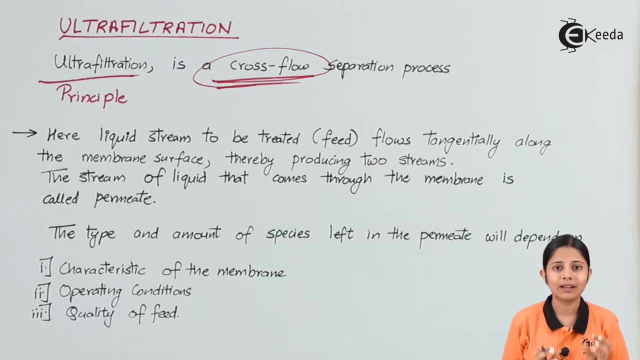 as cross flow separation. That means there are flow of liquid containing certain ions, certain molecules and certain colloidal substances. Now, what exactly are colloidal substances? If I have a water sample which contains colloidal impurities, Colloidal impurities are those impurities which will have 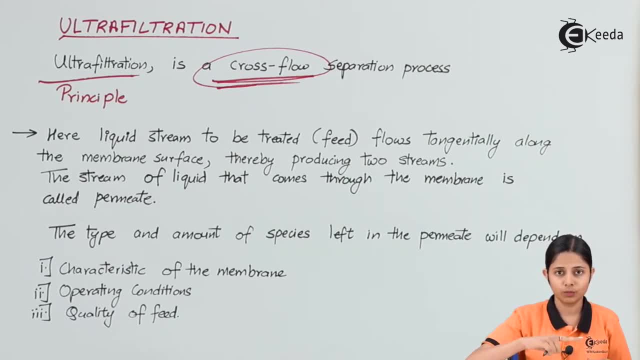 a certain charge on them. For example, I have a negative charge impurity over here and negative charge impurity over here. Both of these impurities are very light and they both have negative charge and that is the reason why, if the upper impurity tries to come down and settle down, it will see. 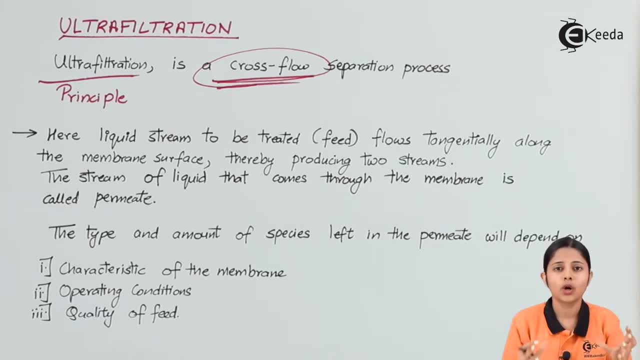 which is down and will repell and go up again. Colloidal impurities are those impurities which are present in water but which will never settle down in water, even after placing water for many hours or days altogether to let the impurity settled on the bottom. and they won't settle down because the 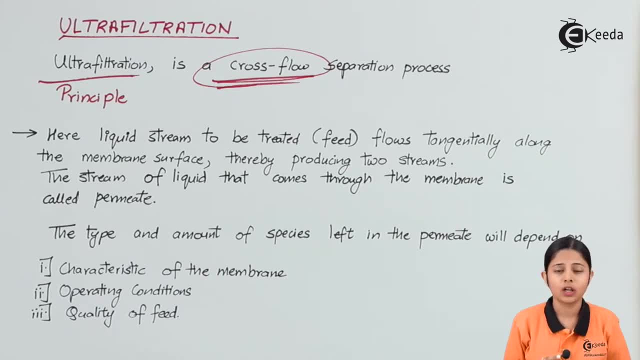 first thing is there extremely light and, if at all, after the weight constraint is taken out, they have charges and because of the charges they either attract or repel each other. and it is done with the water source and use the horas맛. интересно, Shaneen can lend you guys a fun lesson we will take. these two tips again in the next нравится. Victoria, I have now given 1 simple first step. you just need to plan an activity and what this is Next I am going to settle down here. Let us start a Sutro first, to summarize what Norsey said and what you tried to do at this point. Before this art�, sit stroam. 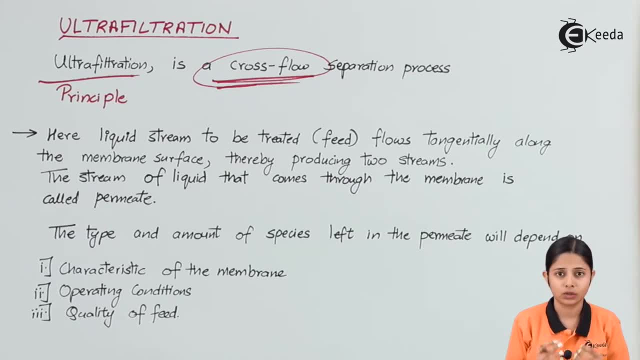 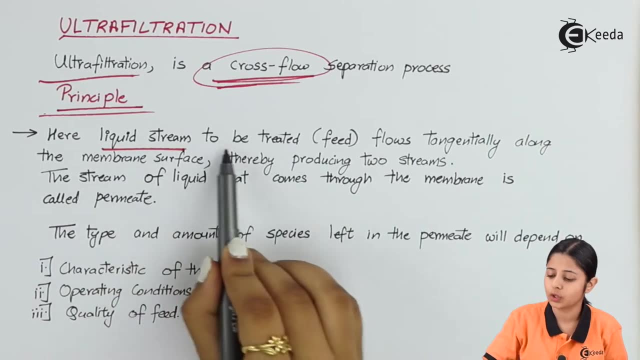 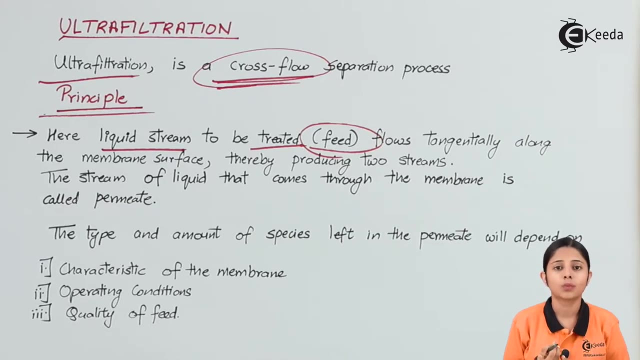 other, and they keep on doing so and remain inside the water rather than settling down. let us see the principle of it: your liquid stream to be treated. that is the field. now feed is the liquid stream that is to be treated, the liquid containing the impurities, the raw. 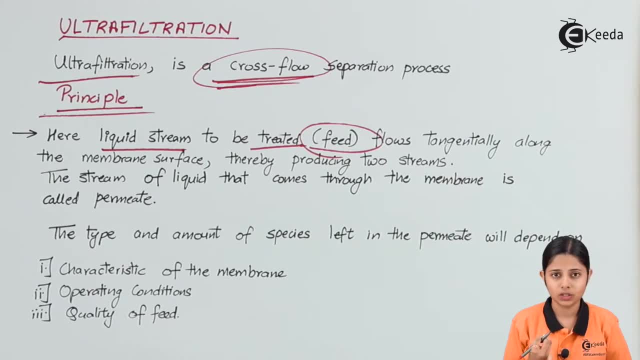 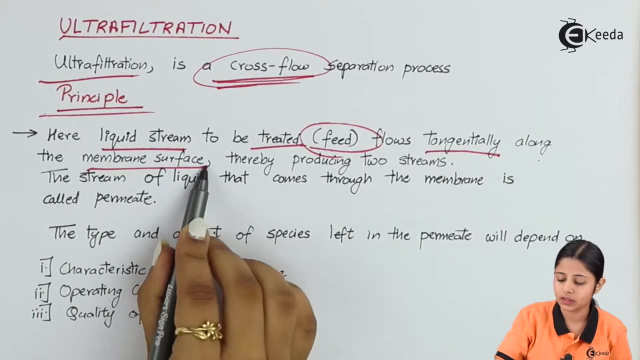 water or the hard water, the liquid which contains ions, the liquid which contains different salts, molecules, metals or colloidal impurities. that is my liquid stream, and it is also known as feed over your flows tangentially through the membrane surface. we'll see this with the help of a diagram. 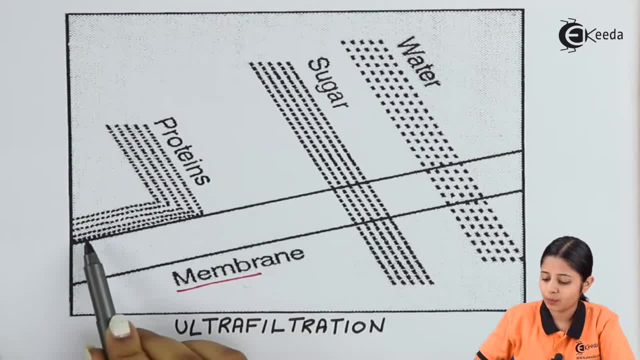 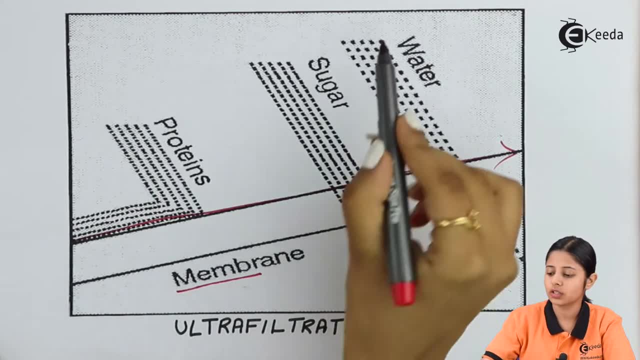 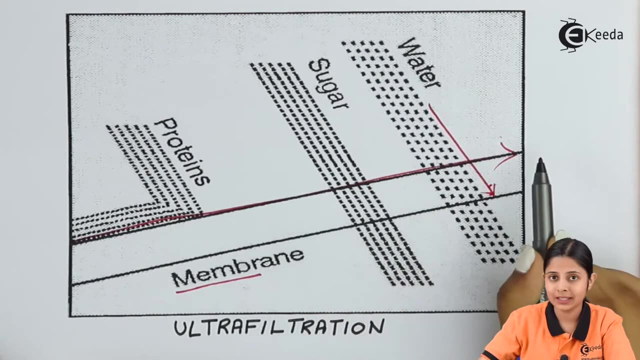 if you see, over here, i have a membrane, this membrane is in this direction and i have my feed, which is coming over here. so this feed is water. so if water is coming over, it is passing tangentially. the flow of water is in this direction, the membrane is in this direction, if i make an angle between: 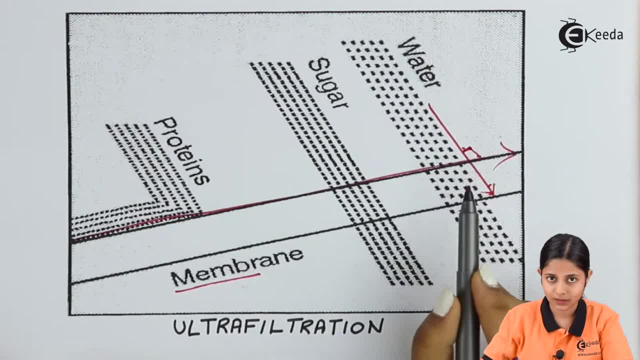 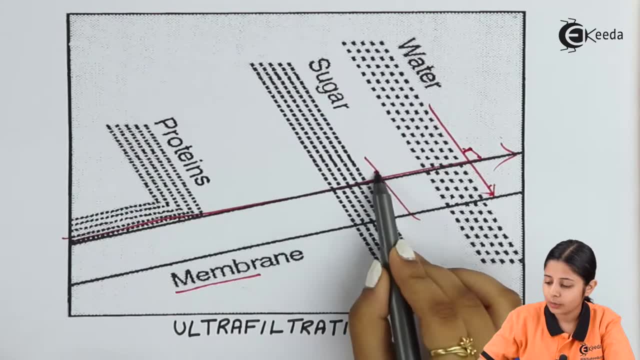 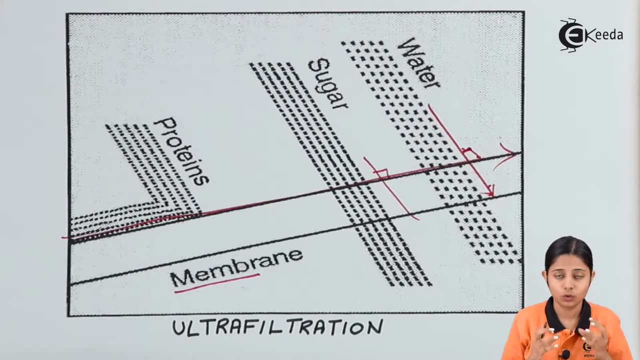 the flow of the water and the membrane, it will be 90 degrees. similarly they have done for sugar. the membrane is going in this direction, sugar is flowing in this direction. if i make an angle, it will be 90 degrees. over here we have proteins. now. proteins are macromolecules. those are molecules. 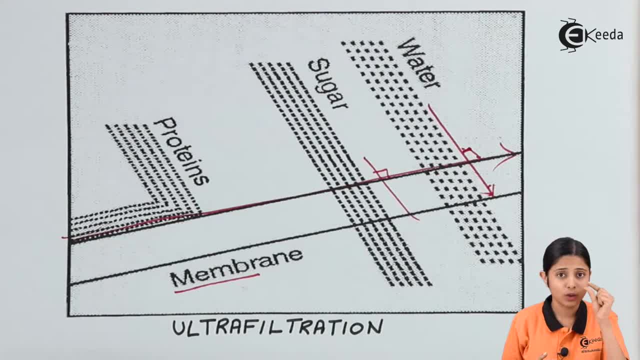 which have high molecular weight, and those molecules are also larger in size as compared to the sugar molecules or the water molecules. and that is the reason why, instead of flowing through the semi-permeable membrane, the proteins are coming over here and then they are going over here. that means they are just flowing parallel to. 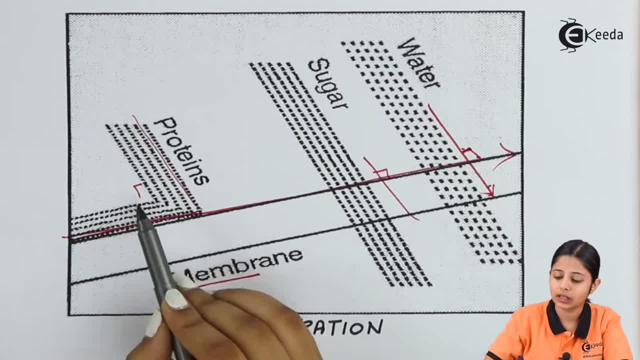 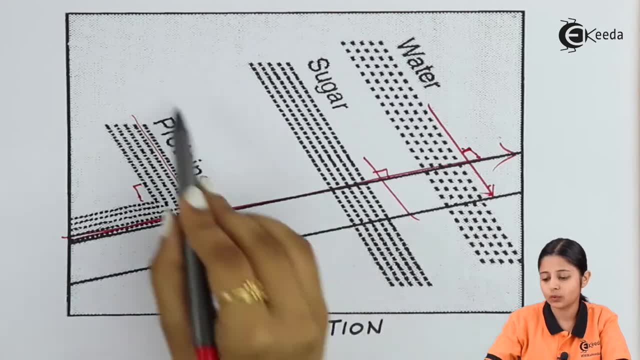 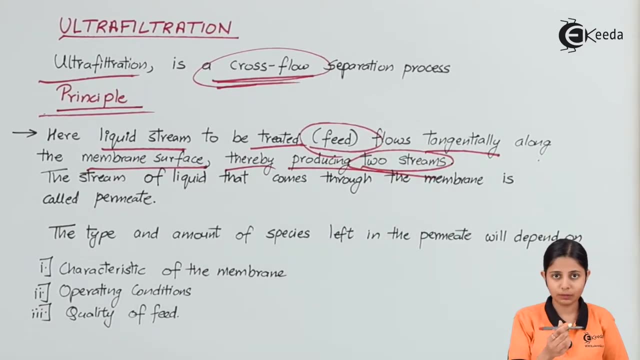 the membrane and they are not passing through it, making a 90 degree over here. this is known as tangential. now let us see what all can pass through the membrane and what all cannot pass through this membrane, thereby producing two streams. now why are we saying two streams? this was my membrane, so if i 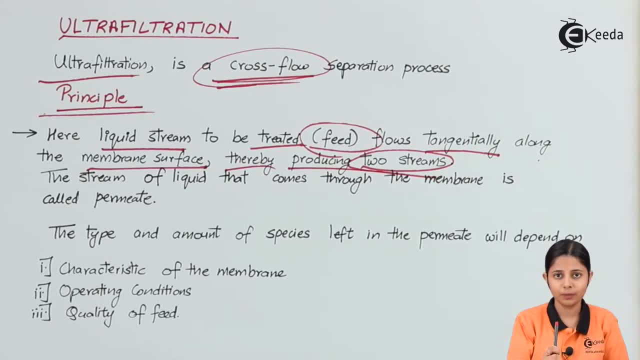 draw a membrane over here. water is passing through it. it's one stream. sugar is also passing through it, making one stream. but protein, when it comes over here, it hits the membrane and goes down like that then then becomes my second stream. this is my first kind of stream which can just 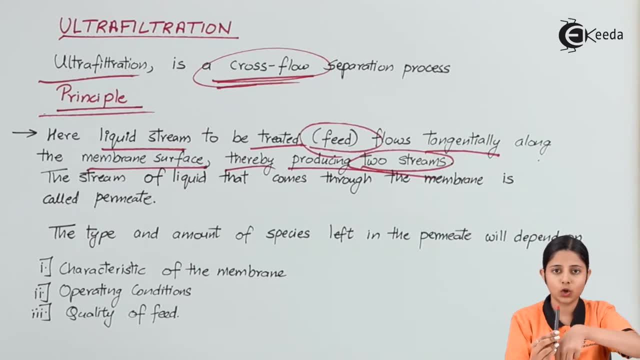 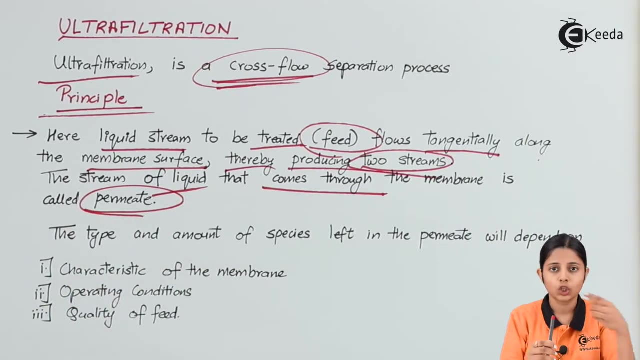 pass through the membrane. and this is my second kind of stream which does not pass through the membrane and goes down, and that is the reason why we have two streams over here. the stream of liquid that comes through the membrane is called as permeate. that means the water which passed through the membrane and came out, the sugar which passed through the. 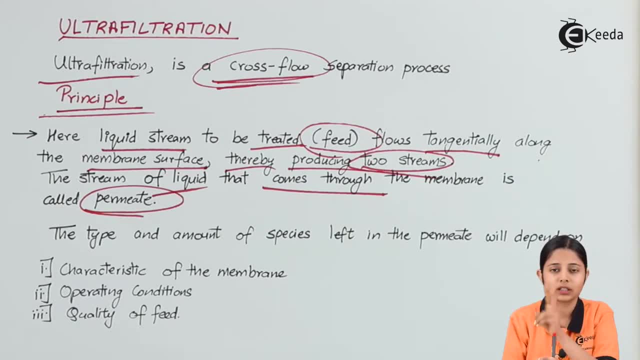 membrane and came out. both of them, which passes through the membrane and comes out in the other direction, are known as permeates. the type of amount of species left in the permeate will depend on. the first is characteristic of the membrane. now, what are the characteristics of? 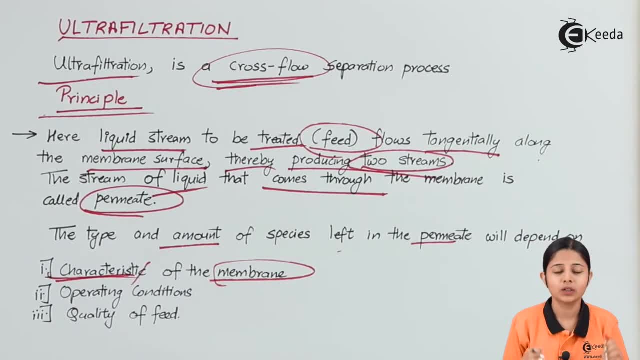 them. the first characteristic of a membrane is the material with which it is made up of. all semi-permeable membrane are made up of certain materials, and those materials decide the amount of pores which will be present in the membrane. those pores help the permeates to pass. 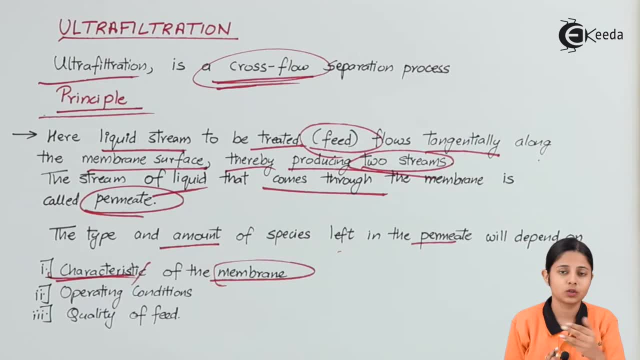 through it. over here the permeates were water and the sugar, which passed through the membrane, but protein, being the bigger molecules, could not pass through it. second is the operating conditions. operating conditions can be the temperature and the pressure. that means if protein is not passing through the membrane, it may. 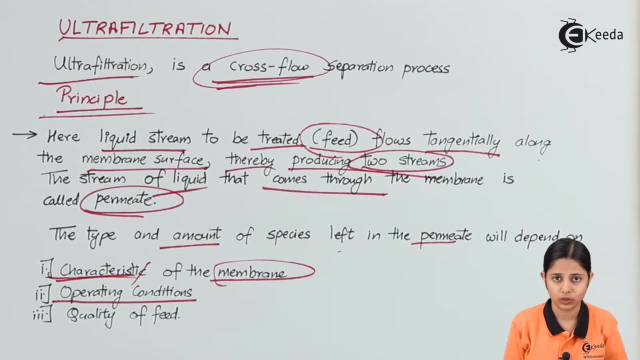 pass through the membrane if we give certain kind of osmotic pressure to it or certain external pressure which is greater than osmotic pressure to it. and the third is quality of the feed. now, the quality of the feed cannot be determined by us, because feed needs to be treated. that is the kind of water which we have, the hard or the 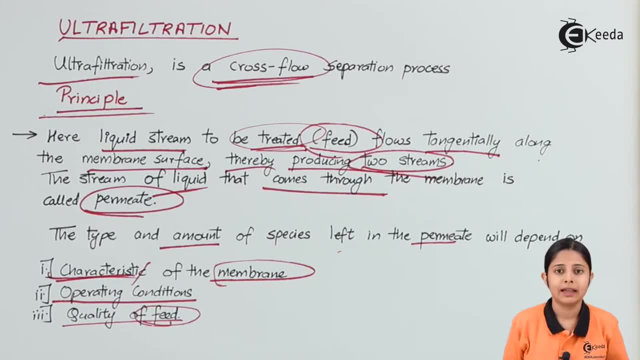 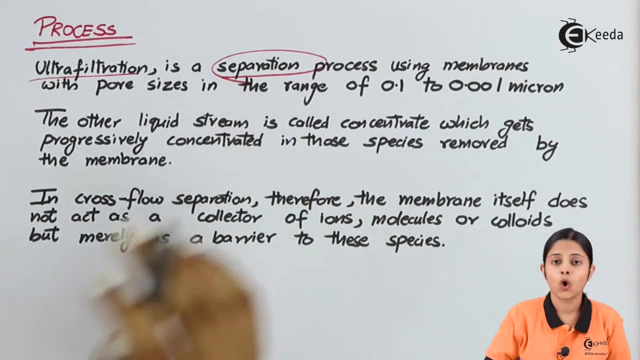 impure water which we have and we have to remove the impurities and that we cannot be responsible for or in charge for. the feed may keep on changing from sample to sample. now let us see the process of ultrafiltration. ultrafiltration is a separation process. 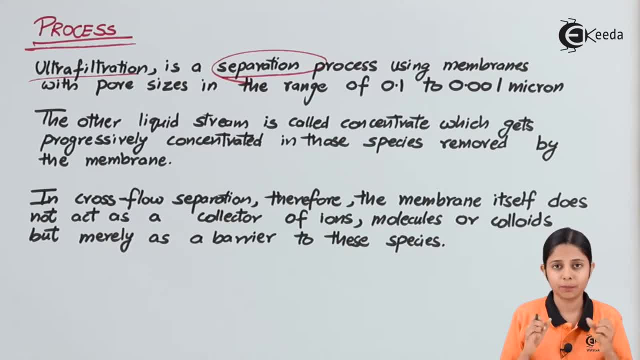 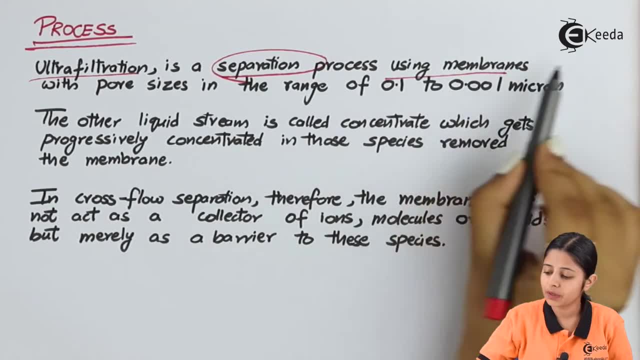 all these processes are separation process, because we need to separate the impurities from the water, and even ultrafiltration is one of them. it is a separation process using membranes. over here the membranes are the semi-permeable membranes, that means the membranes which are made up of certain 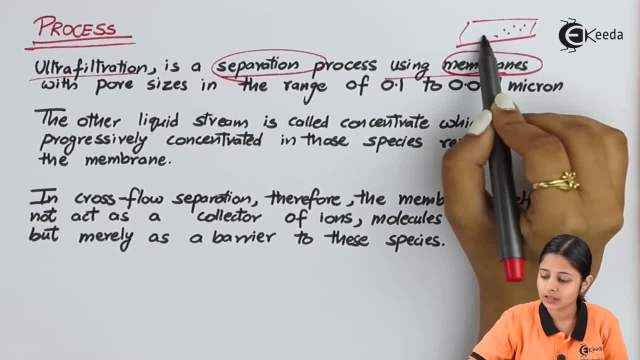 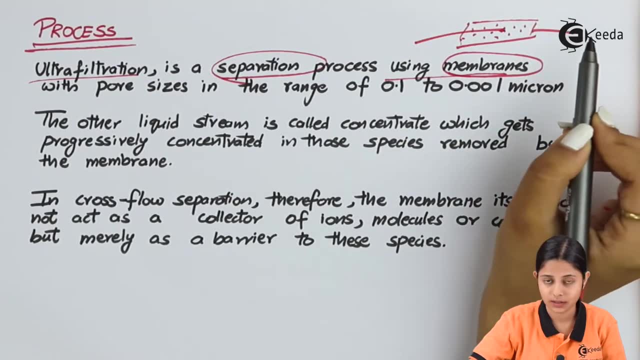 materials and have certain amount of pores present inside them, and these pores will help in passing off the impurities. so this is the process of ultrafiltration. now let us see the process of ultrafiltration of the impurities, or the permeates, from one side to the other side. 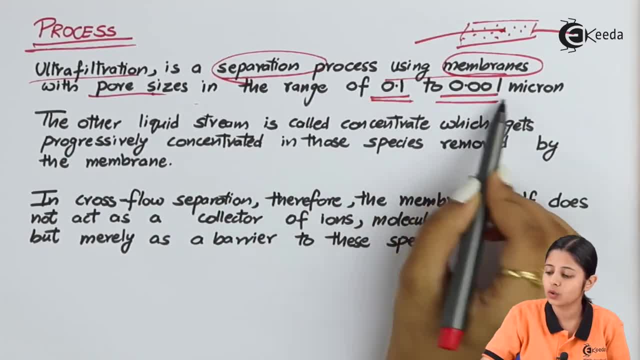 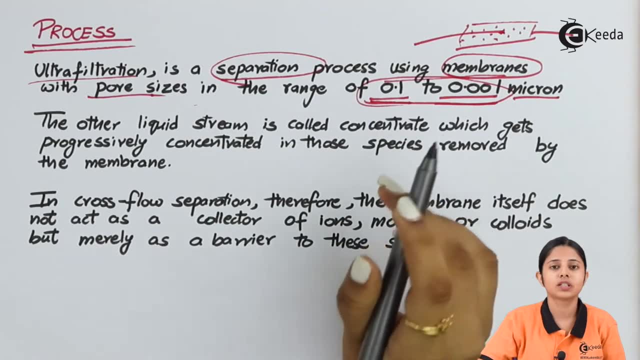 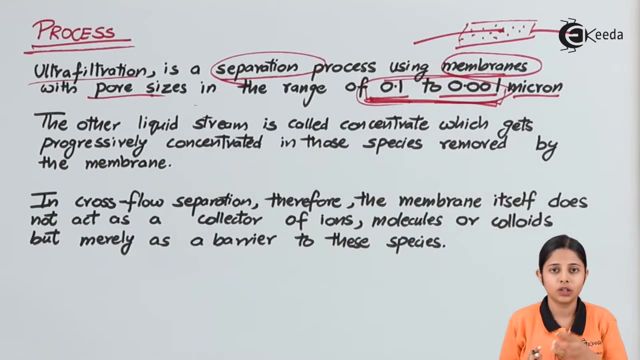 with pore sizes in the range of 0.1 to 0.001 microns. now, this 0.1 to 0.001 is the range of the pore size. we can choose the semi-permeable membranes which are present in this range for. 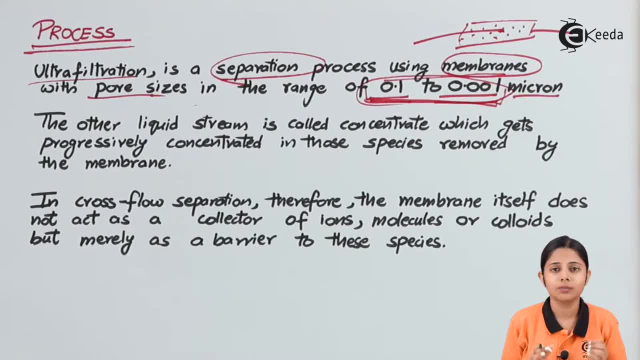 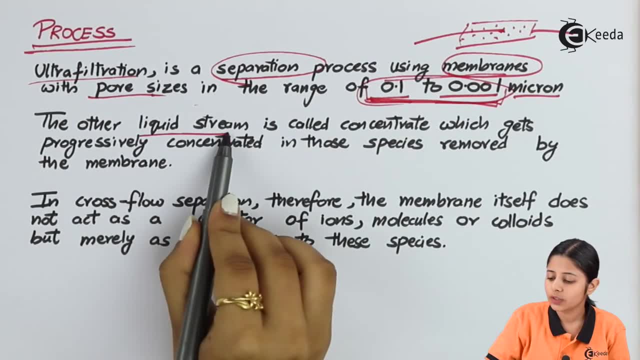 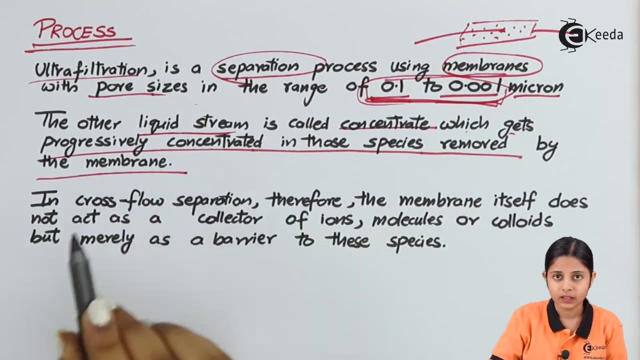 ultrafiltration processes and filter out the ions, the colloidal impurities, the molecules or certain, with the help of these semi-permeable membranes. The other liquid stream is called as concentrate, which gets progressively concentrated in those species removed by the membrane. Now let us see. 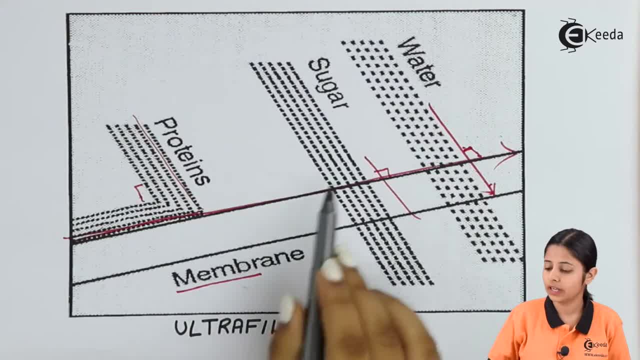 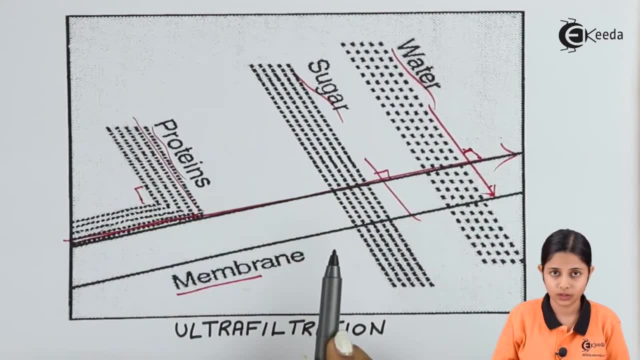 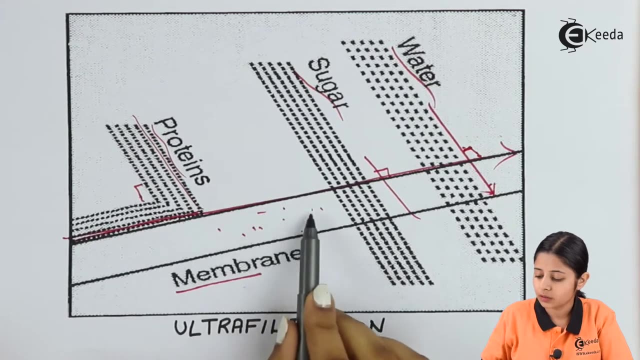 this with the help of the diagram Over here. in the example, we have taken a water stream. This water stream consists of water, it consists of sugar, it consists of protein. Now, over here, this is my membrane and this membrane contains certain pores in it. This membrane contains certain pores. 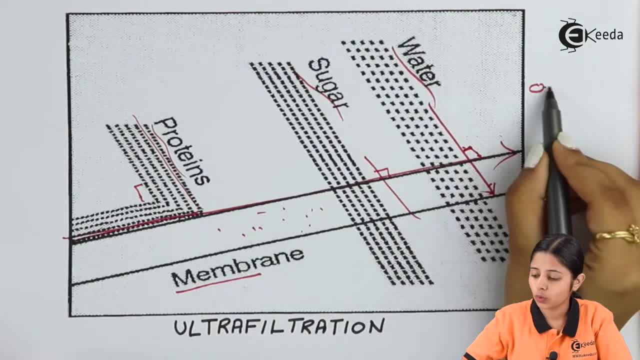 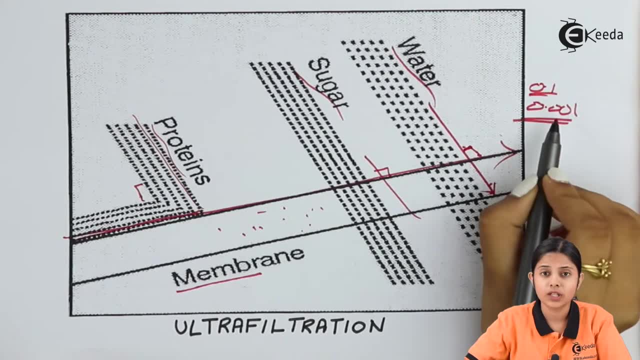 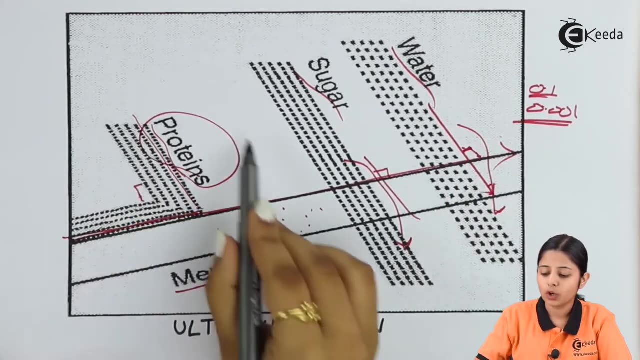 in it. Now. this pores are as big as 0.1 to 0.001 microns. Because of this size, only the water molecules and the sugar molecules could pass through them. The protein molecules which are present in the raw water- that means the protein molecules which are present in the feed- could not. 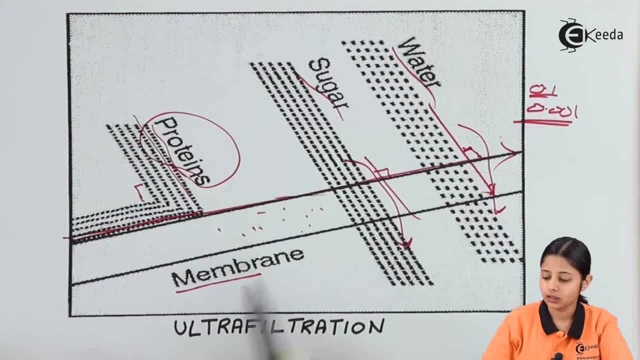 pass through them, And so, once the entire process is done, the water will be a permeate, sugar will be a permeate. What are permeates? Permeates are those which can pass through the membrane. So the water will be on this side, sugar will be on this side. both of these will be permeates, and the concentration of 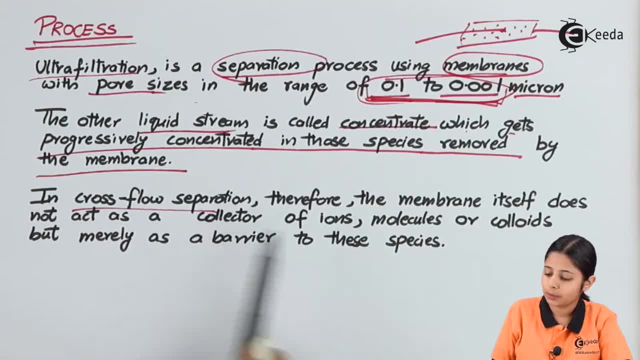 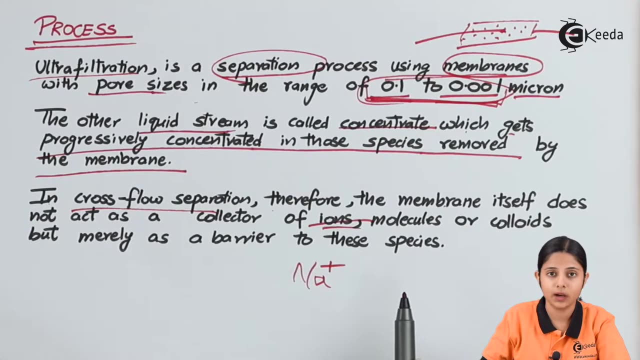 proteins on this side will increase In cross flow separation. therefore the membrane itself does not act as a collector of ions. Now, what exactly are ions? If I am writing Na over here, Na becomes my atom. But if I make a positive charge on it, it becomes my sodium ion. Cl itself is an atom, but if I make a negative? 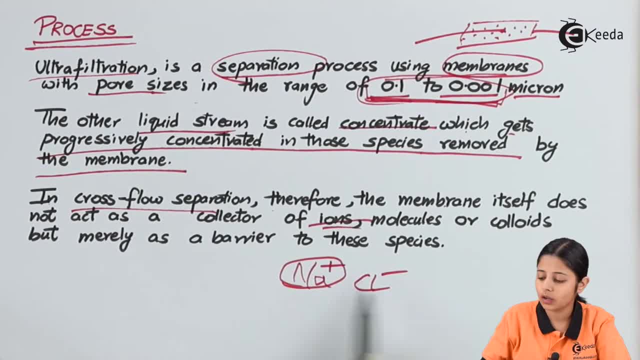 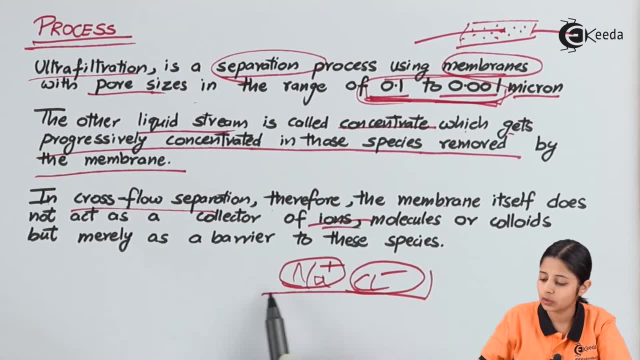 charge on it, it becomes an ion. This is a positive ion. this is a negative ion. Positive ions are known as cations, Negative ions are known as anions, and both of these together are known as ions, which are present in the water and which may contribute to the hardness of the water. In the same way, we 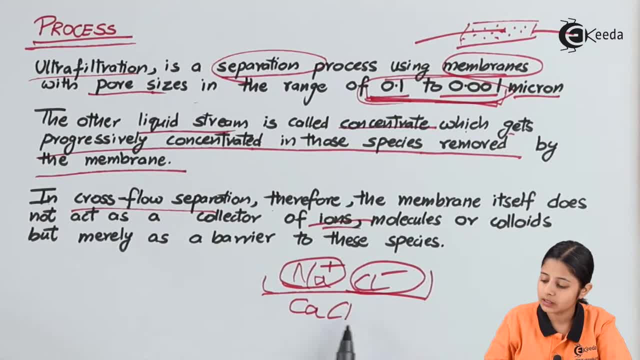 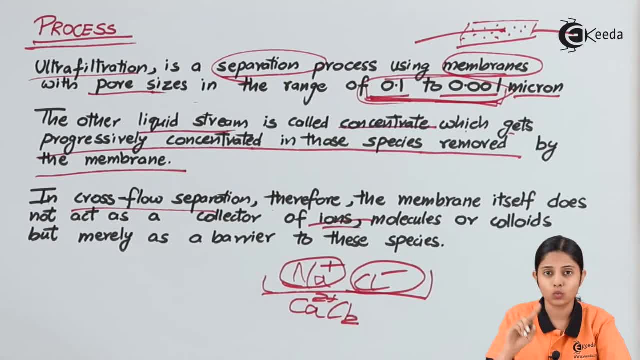 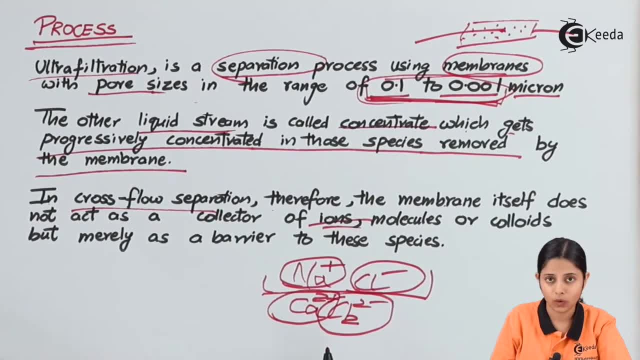 have Cl2 over here, 2 minus. This Ca 2 Plus is a positive ion and over here I have 2 chlorine negative ions. If CaCl2 is present in water, that means I have ionic impurity present in water because CaCl2 will dissociate itself into Ca2 Plus and 2 Cl1 Minus. 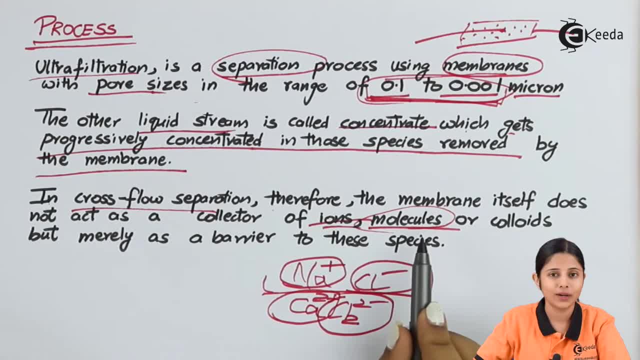 Different molecules which are present in water. now these molecules can be organic molecules or inorganic molecules. over here we had an example of sugar. now sugar in the form of glucose can be c6, h12, o6. c6, h12- o6 is a big molecule and again it 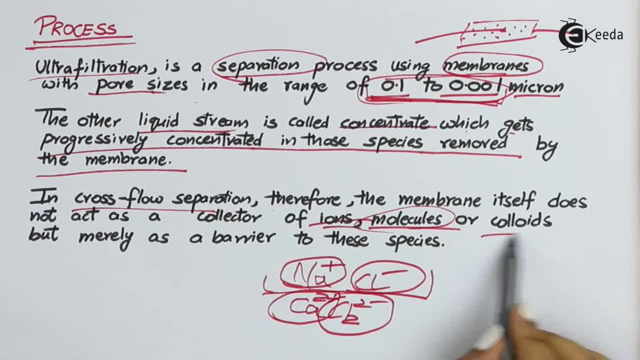 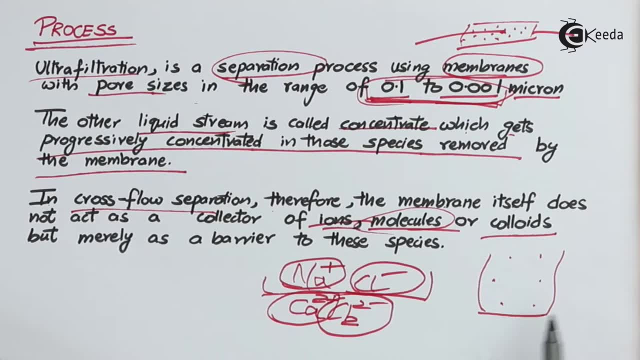 is a molecule. it is not an ionic impurity or colloids. colloids are nothing but small particles with charges. so if i have a water container over here and i have colloids over here, this is a negative charge and over here also, this is a negative charge, if this negative charge wants. 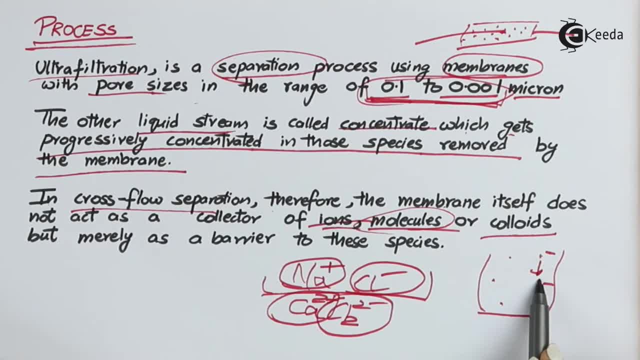 to settle down over here. it will come down, but as soon as it comes in contact with this negative charge, there will be a repulsion taking place between this and this and because of that it will go up again. and so if i have colloidal impurities present in my water and i let that 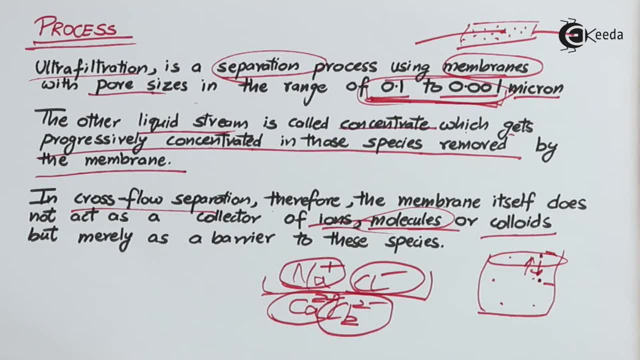 water stand for hours or days, the colloidal impurities will never settle down at the bottom because they will just keep on floating and reacting with each other, either attracting or repelling, because colloidal impurities also contain charges on them, you. but merely as a barrier to these species, let us see the advantages of ultra filtration. 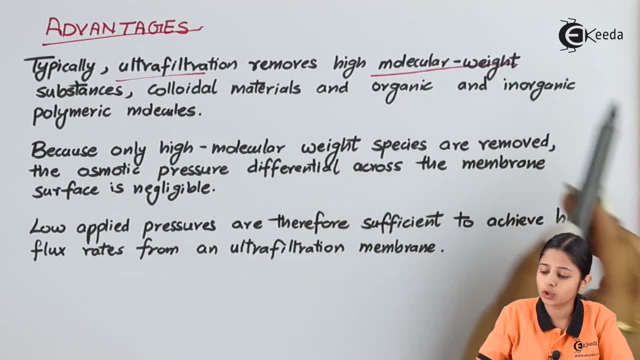 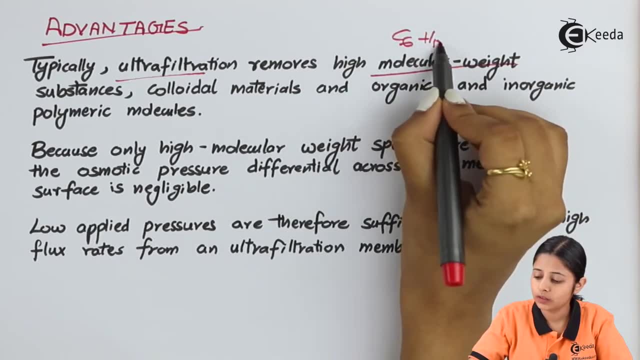 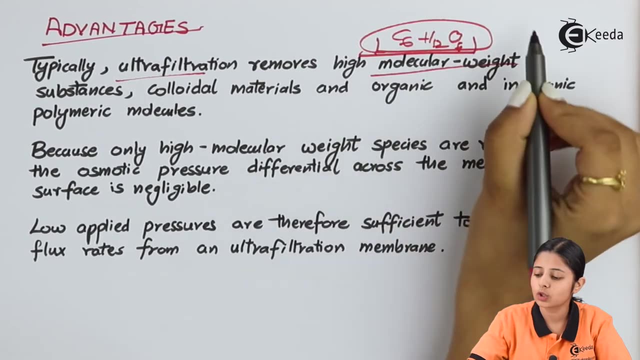 typically, ultra filtration removes high molecular weight substances. over here we had an example of sugar. sugar is nothing but c6, h12, o6, and c6- h12- o6 is a big molecule. but this molecule can also pass through the membrane because we are making it or targeting it tangentially. and since it passes, 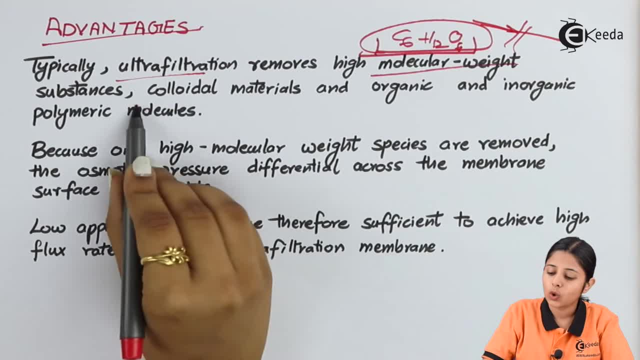 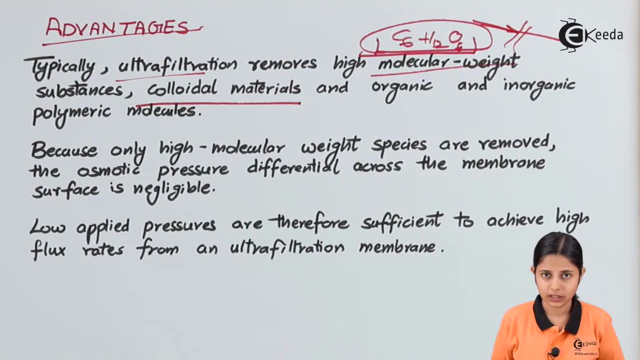 through the membrane, it becomes a permit over your colloidal part materials. all the colloidal materials are small particles containing some amount of charges on them are known as colloidal materials and organic and inorganic polymeric molecules. now what exactly are organic molecules? organic molecules, other molecules which contain a lot of amount of carbon in them. 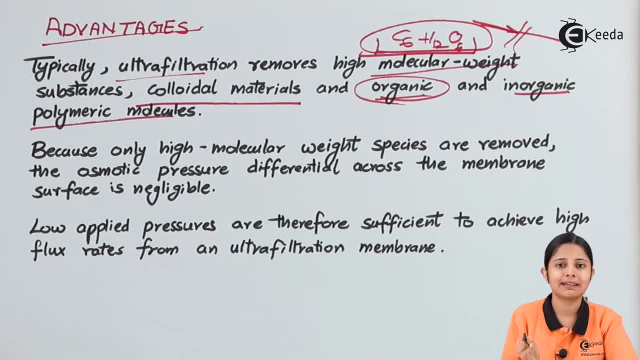 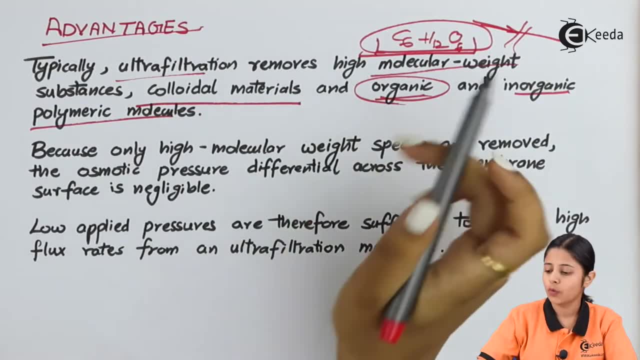 all the hydrocarbons are organic molecules, so aldehyde, ketones, acetones, alcohols, all acetone. Iranianiviram diagram, which we fill in here, the noene Hosth Sil. all of these come under the organic form. Over here we are taking an example of sugar that is: 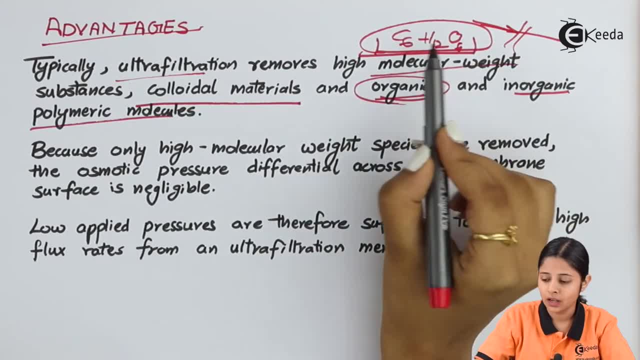 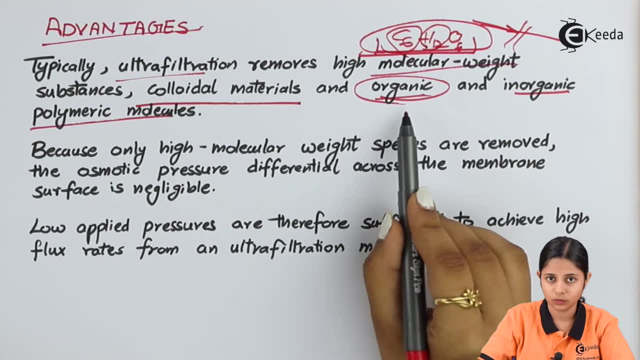 C6H12O6.. It is an hydrocarbon because it contains hydro, that is, hydrogen, and carbon, which is carbon, and thus it is also an organic molecule. Other inorganic molecules. inorganic molecules are those molecules which do not contain any carbon in them, For example, NaCl, sodium and chloride. 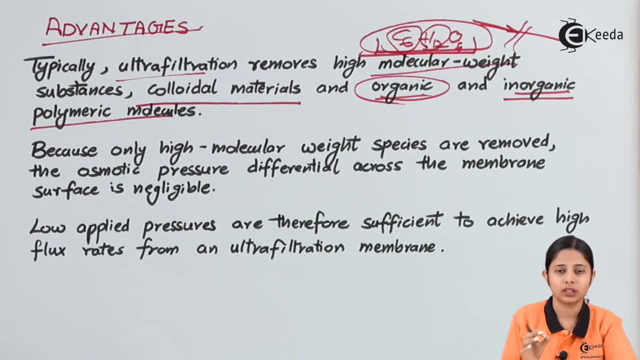 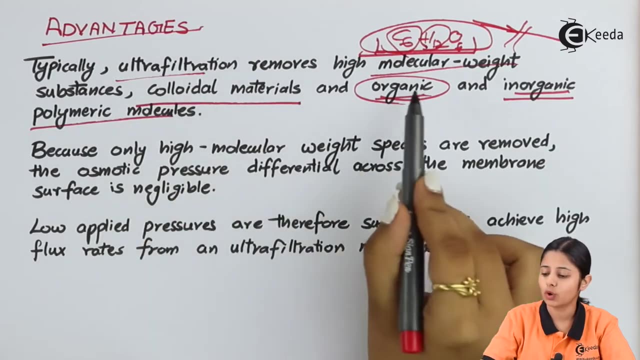 NaCl is an inorganic molecule. AgNO3, silver nitrate, AgN and oxygen- all the three are inorganic. That means there is no carbon and hydrogen added to it, and thus these are inorganic polymeric molecules. Ultrafiltration process is the process which can remove organic as well as 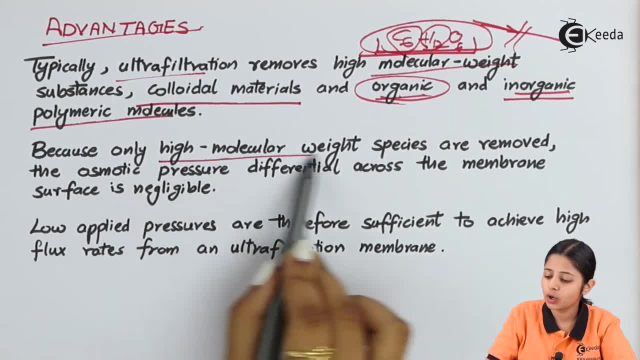 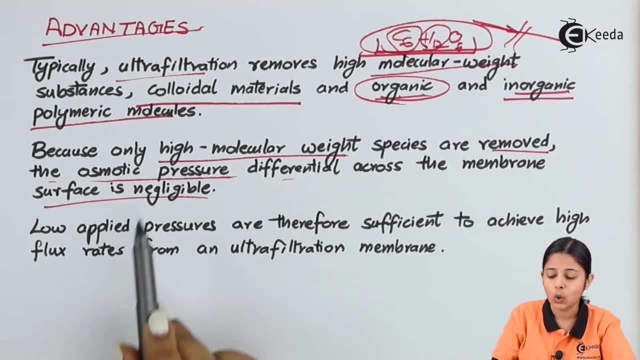 inorganic molecules from it. Because only high molecular weight species are removed, the osmotic pressure differential across the membrane surface is negligible Over here. all the high molecular weight species are removed. Proteins are removed. sugar is removed, all the molecules containing many elements in it. a large amount of atoms in it are high. 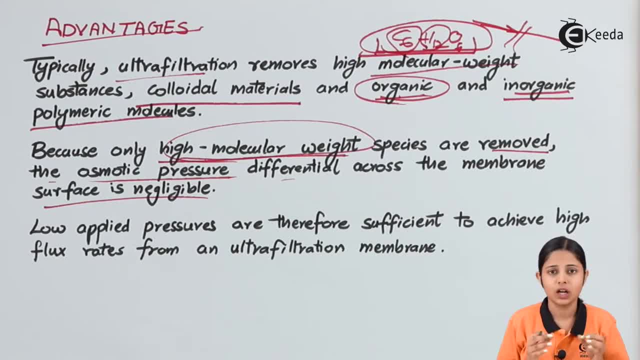 molecular weights, and all of them can be easily removed by using the ultrafiltration process. because it uses the cross reference of water, Differential across the membrane surface is negligible. Low applied pressures are therefore sufficient to achieve high flux rates from ultrafiltration method. Over here I have a. 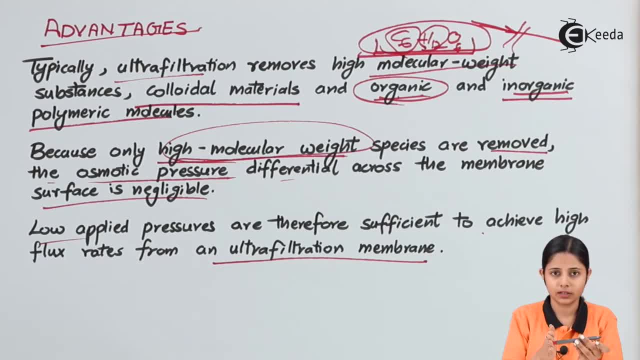 membrane over here and the water, and this because of this, 용 appear and because of this, because of this it is tangential and thus we do not have the need to apply a lot of pressure, and that is not the case in other filtration. so placing here 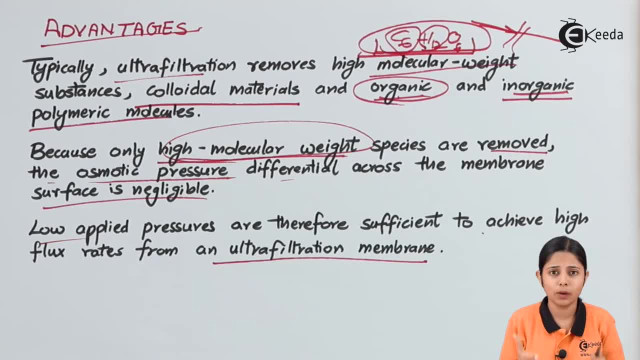 hyper filtration or reverse osmosis. also use using cross reference term or reverse osmosis. there we need to apply certain kind of external pressure or we need to apply certain kind of change in temperatures, but in Ultrafiltration none of them are needed. Now let us see the 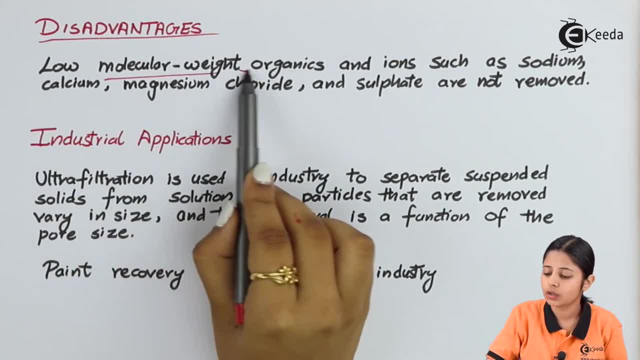 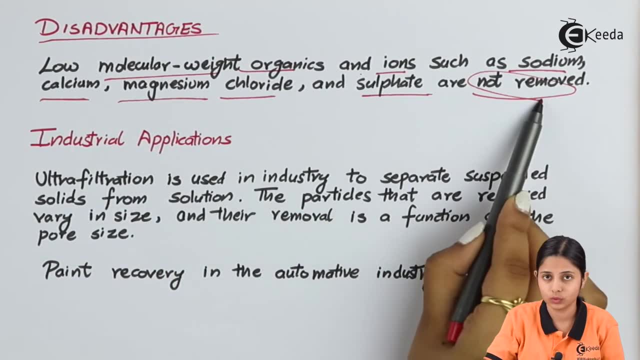 this advantages of it. now lets Low molecular weight no hard. latest, the those omega in omega violate a hypovlungal protein protein. fast to much change. basically, kam Shop, give me not word organic and ions such as sodium, calcium, magnesium, chloride and sulfate are not removed. 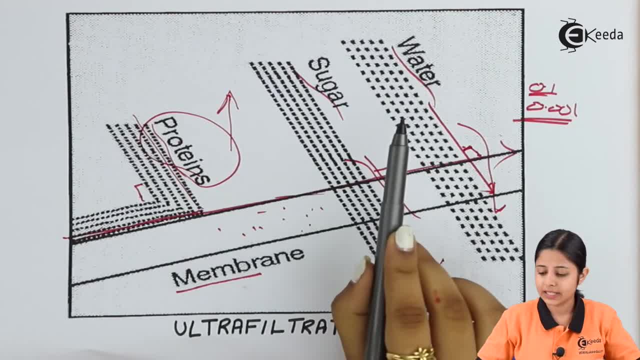 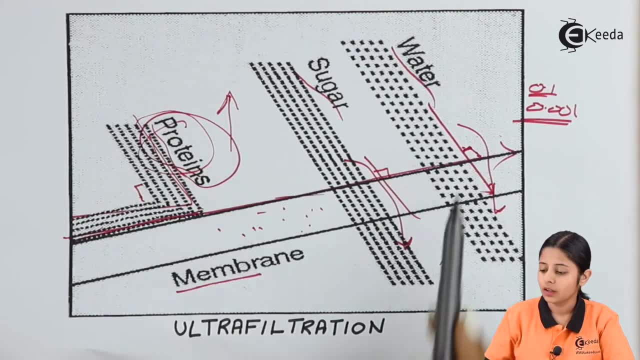 Let us see this with the help of a diagram. So over here, if we see the diagram, we could see the proteins which were there, which were impurities, just went away, could not pass through the membrane, but over here there was water and the water passed through the membrane easily. There are many. 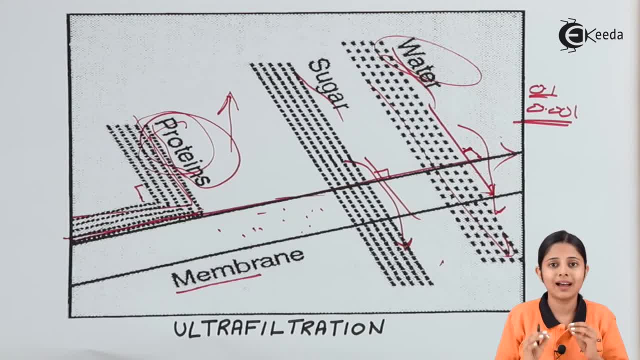 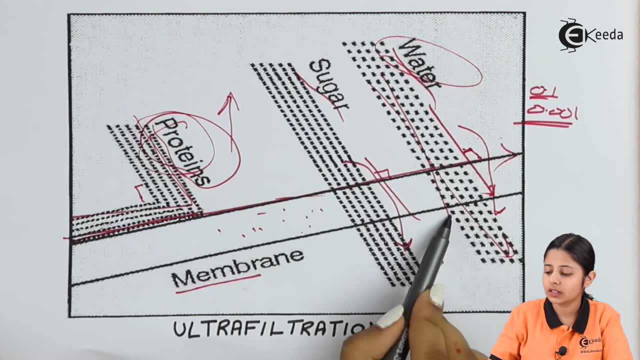 dissolved salts in water, and all these dissolved salts are a part of water and that is the reason why all the dissolved ions will pass through it very easily, and this is what they have said: in the disadvantage When water can pass through such easily. that means H2O molecule, the entire molecule. 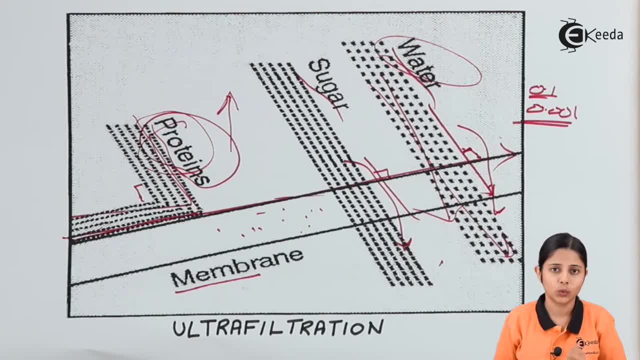 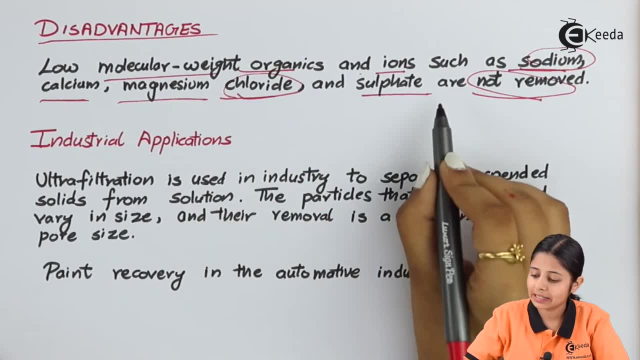 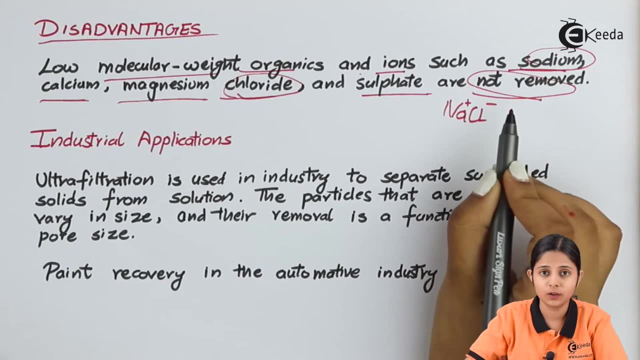 can pass through so easily. Small ions can also pass through it as well. So when they are talking about the sodium and the chloride ions, the example can be NaCl. So if I have dissolved NaCl, it is possible that some NaCl ions will be filtered out, but some NaCl ions will still be. 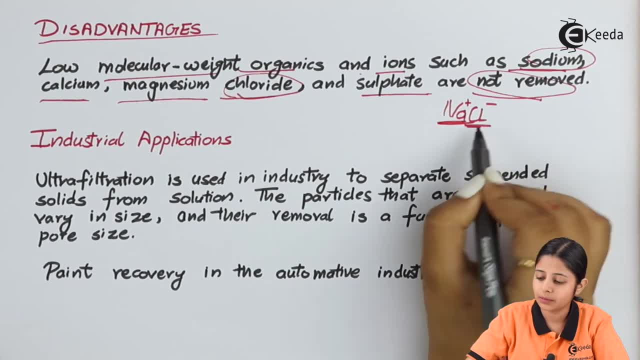 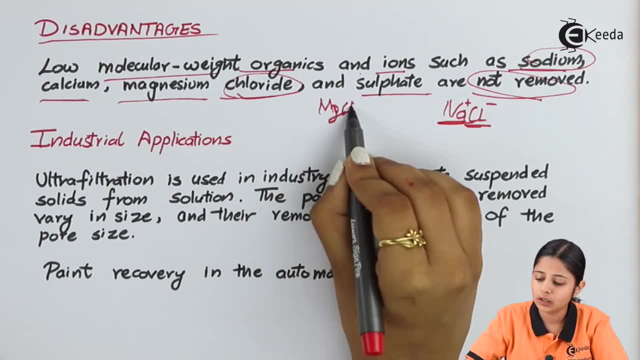 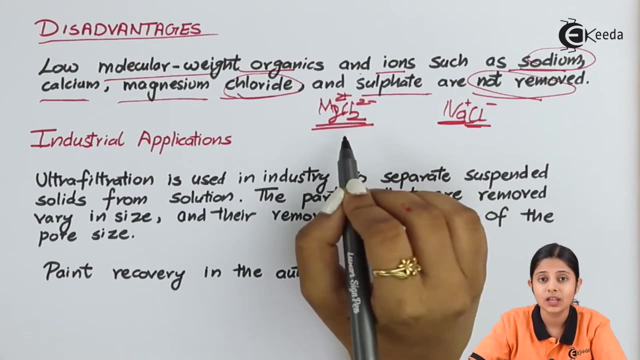 in the permeability. So Na plus becomes my sodium, Cl minus becomes my chloride, Even magnesium and chloride forms MgCl2, and if I have MgCl2 present in the water I will have Mg2 plus and Cl2 minus again. there is a possibility of these ions passing through the permeate and being there in the filtered water. 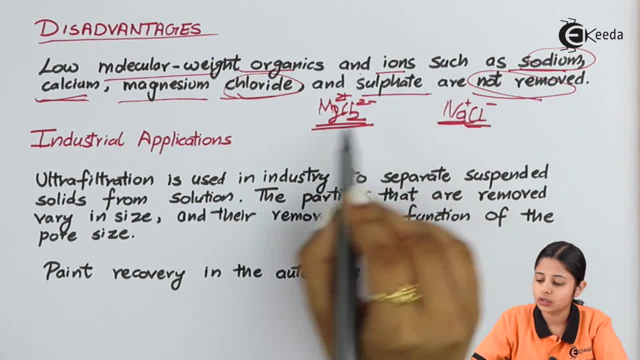 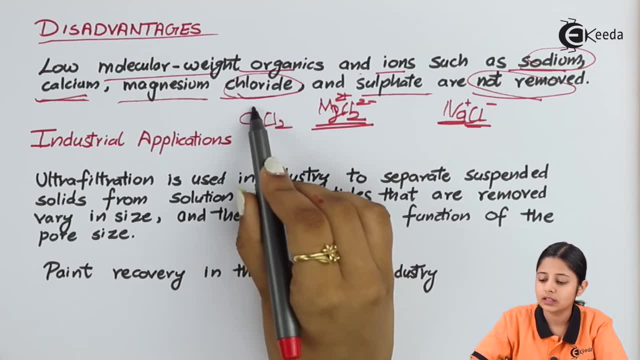 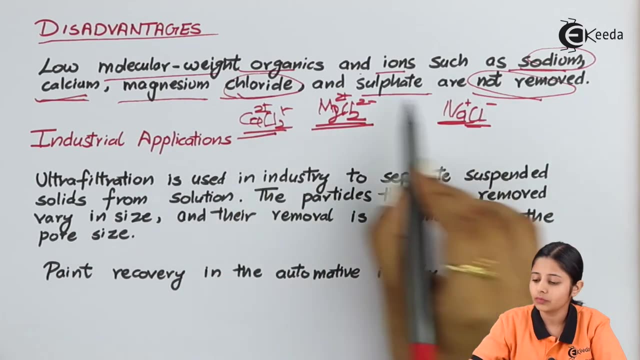 form. There is calcium and chloride as well, so this can be CaCl2.. If CaCl2 is dissolved in water, then Ca2 plus ions and 2 Cl1 minus ions are present in water, which may pass through the permeate. Then we have sulfates, Sulfates of calcium, sulfates of magnesium. Sulfates of calcium can be CaSO4.. 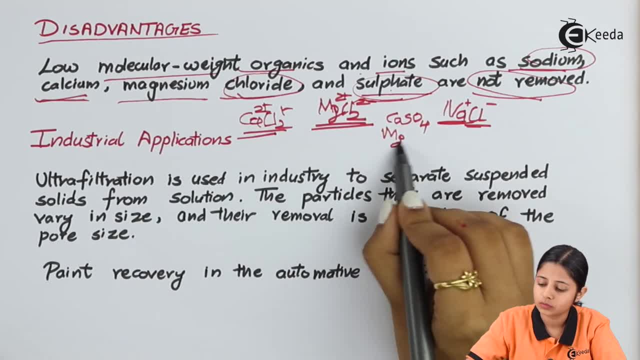 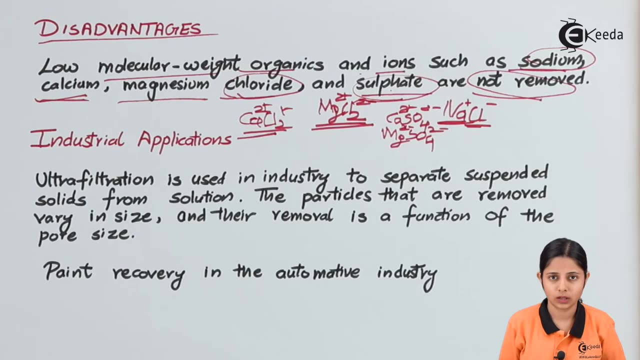 Magnesium sulfates can be MgSO4. Again, Ca is 2 plus SO4 is 2 minus. Mg is 2 plus 2 plus SO4 is 2 minus. So from CaSO4, I can have 1 Ca2 plus ion and 1 SO4, 2 minus ion In MgSO4,. I can have 1 Mg2 plus ion and 1 SO4 2 minus ion. Now these are comparatively small and maybe there are chances of passing through the membrane, through the pores of the size 0.1 to 0.001 microns. Let us see the industrial application of this ultrafiltration method. Ultrafiltration.